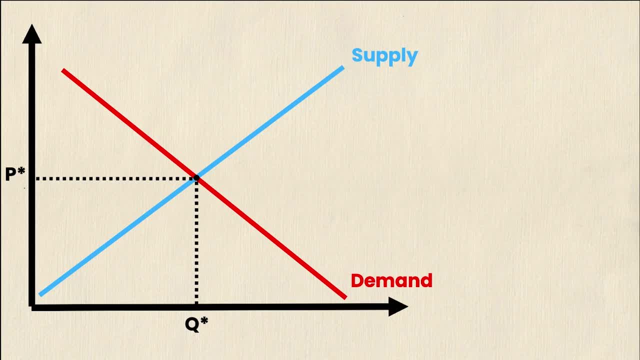 equilibrium price is too low, it can impose something called a price floor. A price floor is a legal minimum that must be charged for a good. Now, in order for a price floor to be effective, or what economists call binding, the price floor must be higher than the equilibrium price. 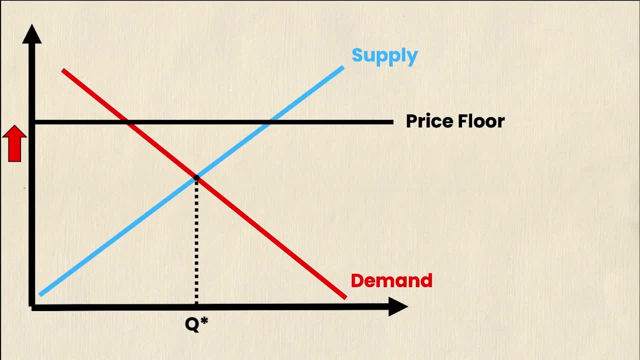 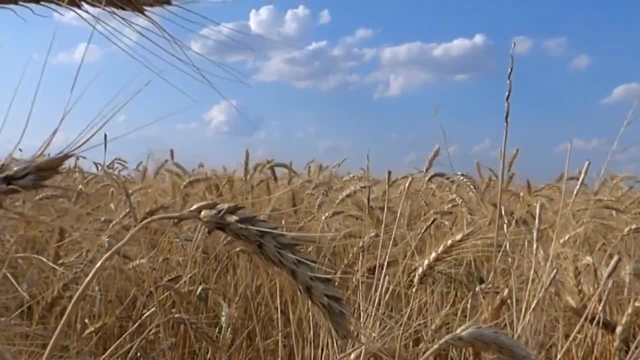 A real life example of a price floor imposed by the government is when they impose a price floor on wheat. This increases the price or the wage that farmers get paid for producing wheat to ensure that they receive at least a certain amount of money so that the toil of farming wheat is. 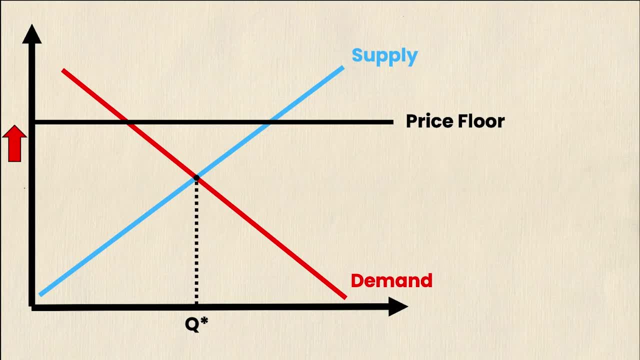 worthwhile, But price floors lead to market inefficiencies. After all, the market is no longer in equilibrium. This will lead to something that economists call a dead weight loss, where both producers and consumers lose some of their surplus. This is depicted by the yellow 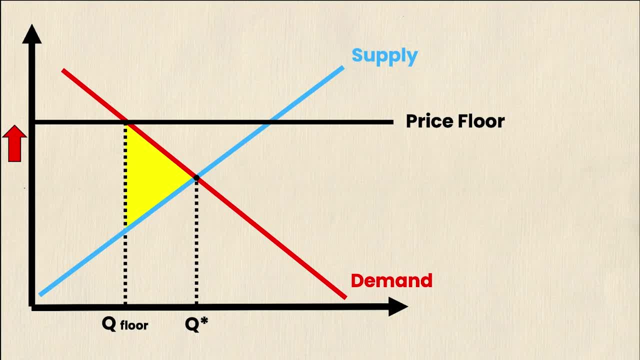 triangle on screen. If you want a detailed video outlining dead weight loss, just let us know in the comments. Price floors lead to excess supply, also known as a surplus, unnecessarily high quality goods and inefficient allocations to producers. In other words, oftentimes price floors end up. 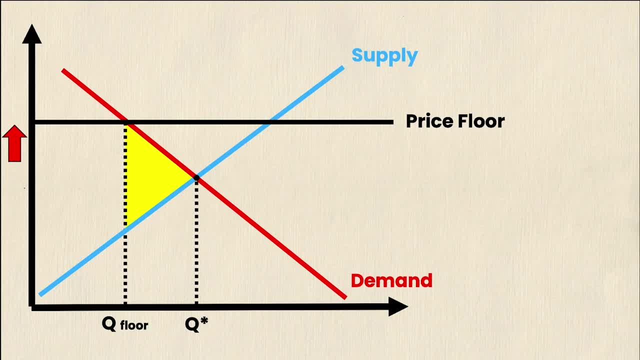 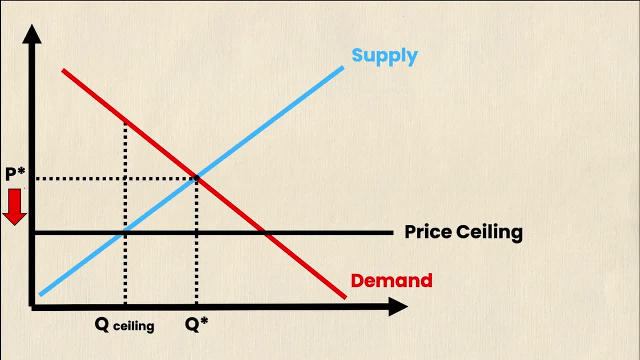 being wasteful. On the other hand, if the government believes that the equilibrium price is too high, they can impose something called a price ceiling, Opposite to a price floor. a price ceiling is the maximum price that can be achieved by the government. So if the government believes that the equilibrium 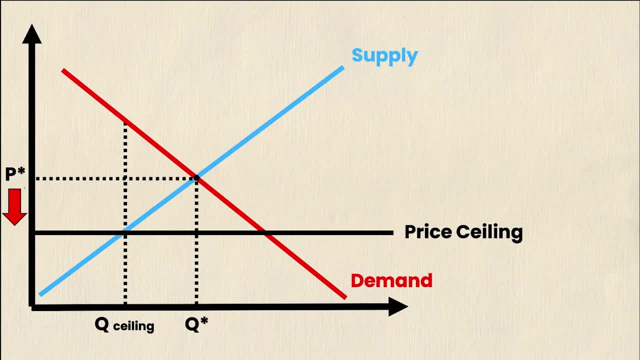 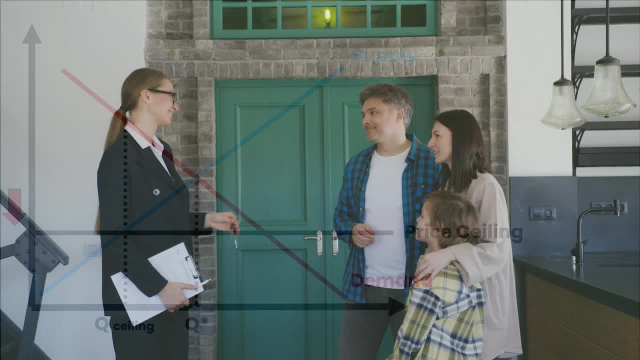 price is too high, then the government can impose a price ceiling that can be charged for a good. Once again, in order for a price ceiling to be effective, or what economists call binding, the price floor must be lower than the equilibrium price. A real life example of a price ceiling is rent control. 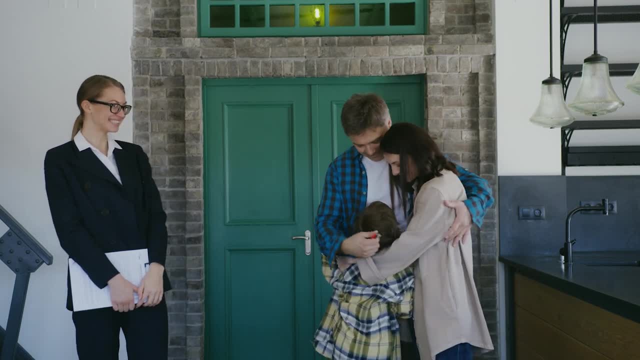 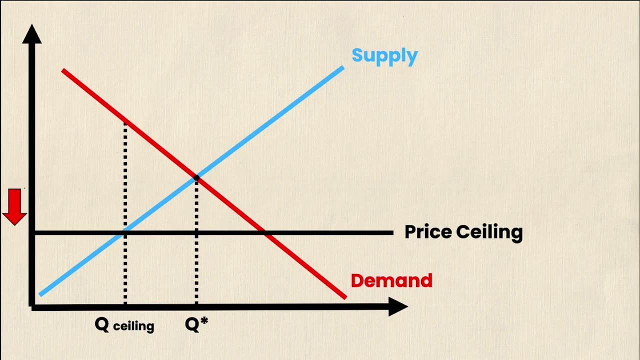 This is where the government limits what landlords can charge for rent or a rental increase, in an attempt to make housing more affordable. However, similar to a price floor, a price ceiling also leaves the market in disequilibrium, creating yet another dead weight loss. Price ceilings lead to excess demand, also known as a surplus. 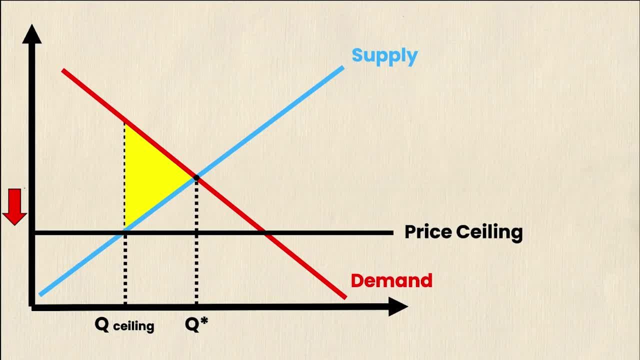 as a shortage, wasted resources, black markets and inefficient allocations to buyers. Now you may recognize that price ceilings and price floors look just like the graphs for shortages and surpluses respectively, And that's because, well, in both cases, government price controls.